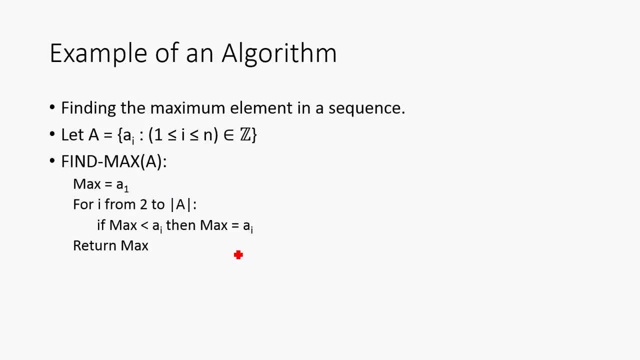 finite and correct. So here's an example of an algorithm. We're going to find the maximum element of a sequence, So let's go ahead and define it. So first we're going to start by passing in A as an input, which is going to be the set here of all the elements in the sequence. So we start off by: 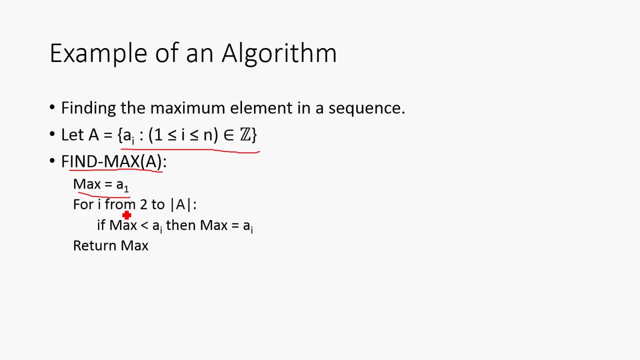 setting the max equal to the first element, And then we go from 2 to the size of A And we're going to set the current element to the max And then by the end we should have our max. so we just return it. So that's an example of an algorithm. 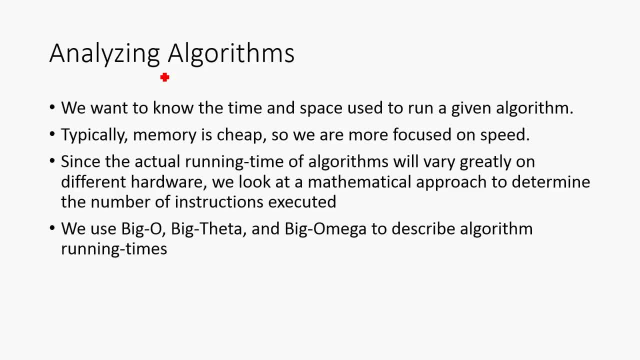 So typically we want to know the time and space used to run a given algorithm. Since memory is usually cheap, we tend to focus more on speed or the time it takes to run it. Since the actual running time of algorithms will vary greatly on different hardware, we'll 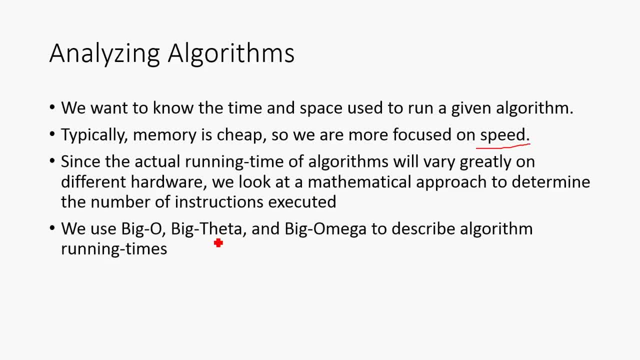 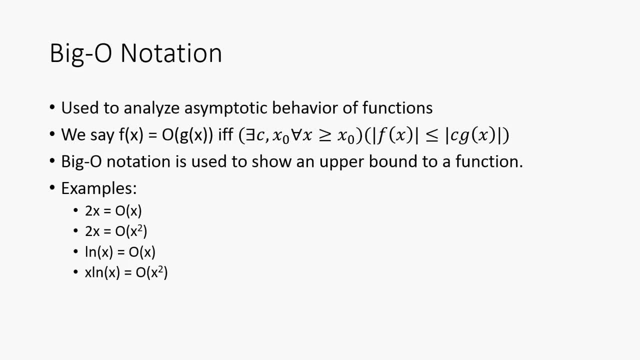 look at a more mathematical approach to determine the number of instructions executed. We tend to use O, theta and omega to go describe how different running times. So this is big O-notation and it's used to analyze the asymptotic behavior at functions. 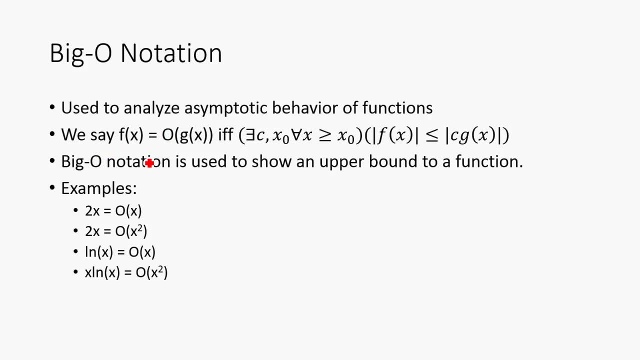 It shows an upper-bound function. so we say that F is O g of X If, and only if, there exist constants C and Xv's such that all x greater than or equal to x-naught, the absolute value of f of x is less than or equal to the. 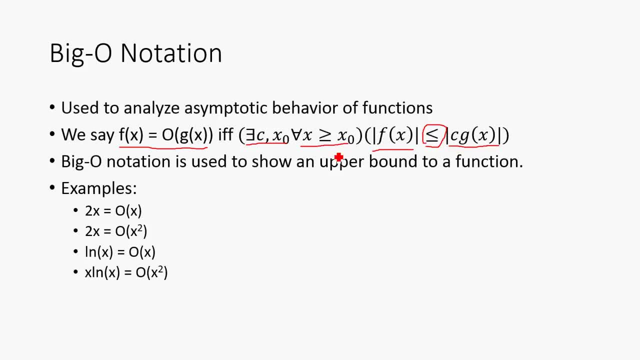 absolute value of c times g of x. so some constant c right, And, like I said, it's used to show an upper bound. so here are a few examples of it being applied. Clearly, 2x is going to be big O of x because it differs only by this constant here, 2.. And we can. 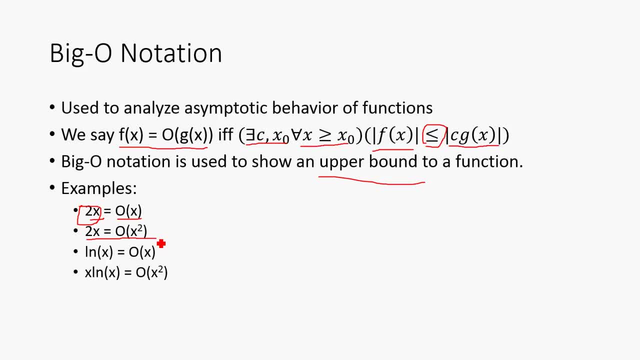 note that 2x is going to be big O of x squared right, Because if we just take, for example, all x greater than, let's say, 2, it's going to x squared is going to be greater than. 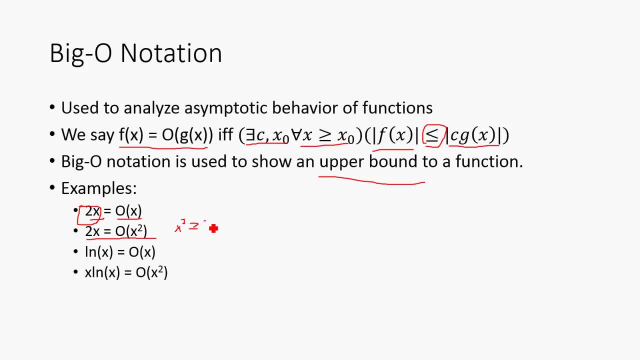 or equal to 2x. right for all x greater than or equal to 2.. Let's take another case: The natural log of x. Let's draw the natural log graph just to see what it looks like. It's going to look something like this. And then x is going to look something like that: 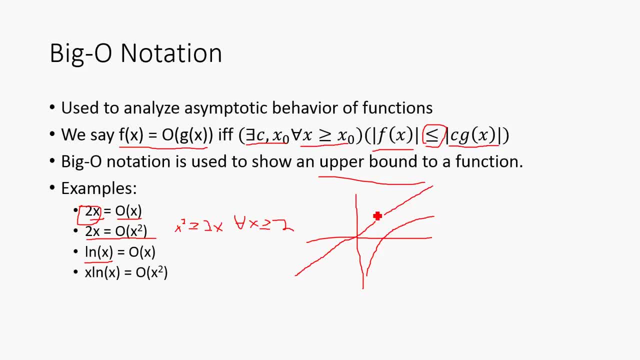 Clearly it's going to be an upper bound to the natural log, And thus if we multiply both sides by x, we can see that x- natural log x is going to be big O of x squared, And this is a key relationship in sorting. 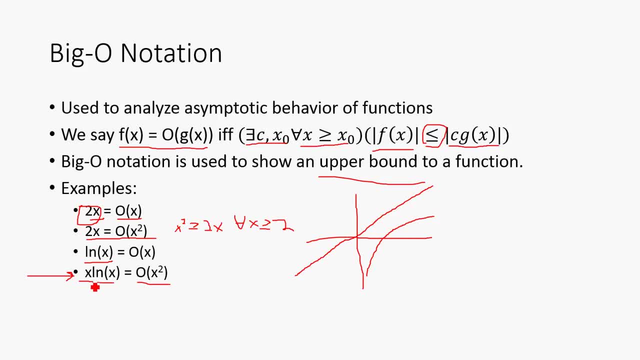 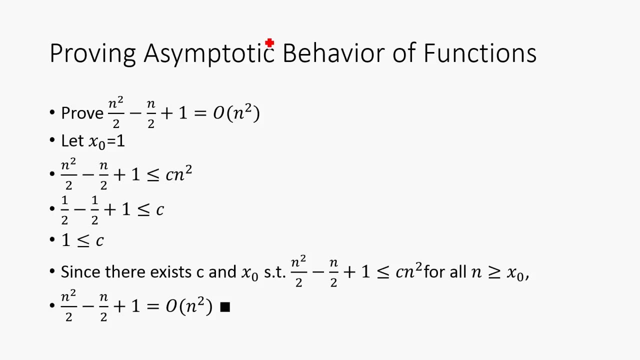 A lot of sorting algorithms have running times of n, log n and n squared, where n is the number of elements in this beta structure that we're trying to sort. So we can use our definition to prove the asymptotic behavior of functions. So, for instance, let's prove that n squared. 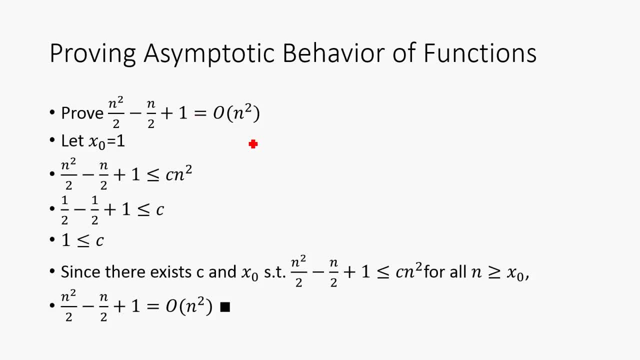 over 2 minus n over 2 plus 1 is big O of n squared, So we're going to let our x not be 1.. we're going to go ahead and solve for c, So we have our relationship right here, and we're going to go ahead and plug in our 1, so that just leaves 1 half minus a. 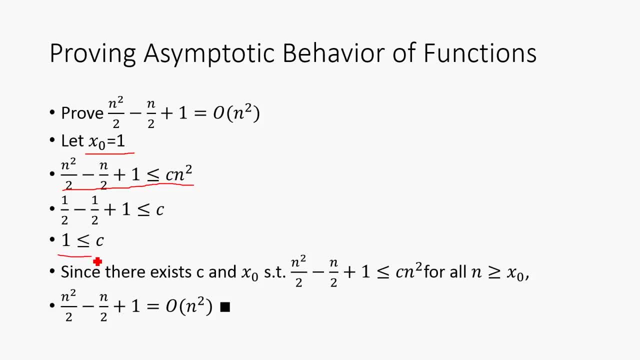 half plus 1 is less than or equal to c. therefore c is greater than or equal to 1.. So since there exists, exists c and x naught, such that this relationship holds true for all n greater than x naught, we say that this first function here is big. 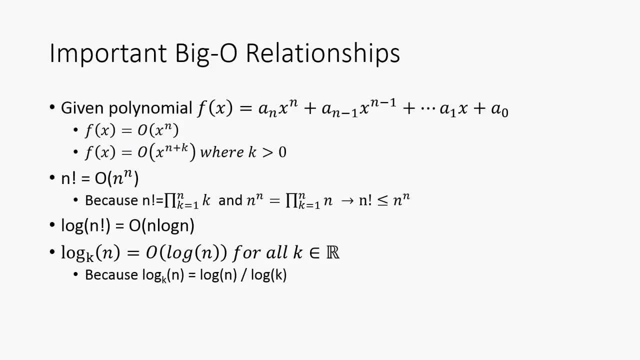 O of n squared thus completes the proof. So an important big O relationship to remember is that, given a polynomial of degree n right here, and whatever constant coefficients are on the terms, we say that f of x is going to be big O of x to the n. 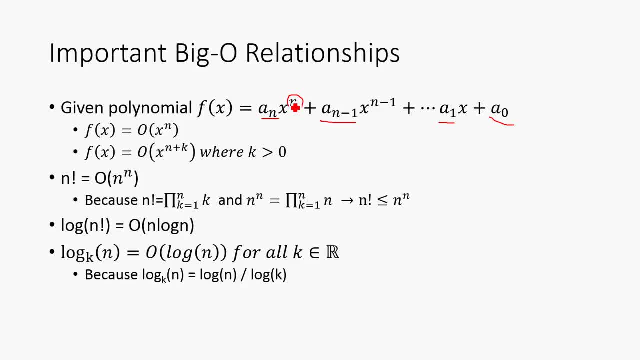 and we also say that this f of x of degree n is going to be big O of any degree polynomial of x bigger than n. So, for instance, x is going to be big O of x squared. That's what I'm meaning by there, And it's also important to note that n 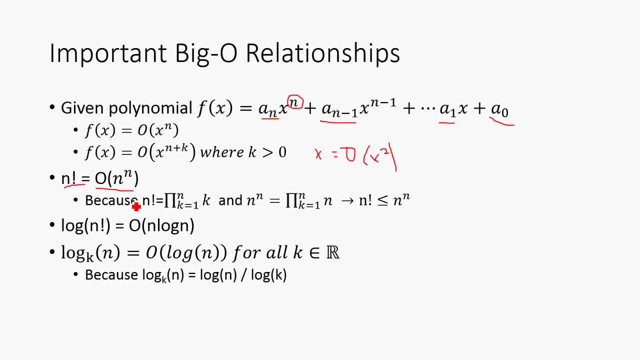 factorial is going to be big O of n to the n right, because n factorial is just going to be the product of the numbers from 1 to n right. So we've got this relationship right here to denote this, where the big pi is simply just like big sigma. So this would just stand for product instead. 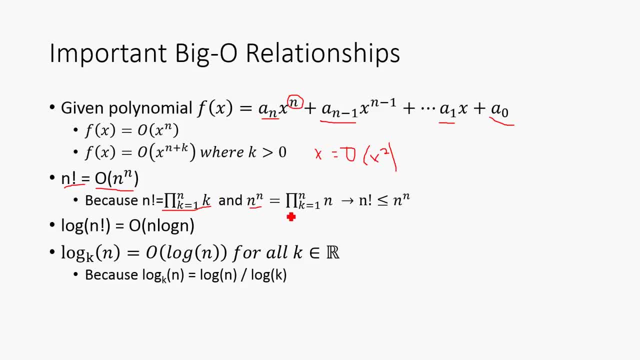 of sum And then n to the n is going to be over the same number of variables, it's just going to be n, which is that upper number. So if we take for all n greater than or equal to 1,, this relationship. 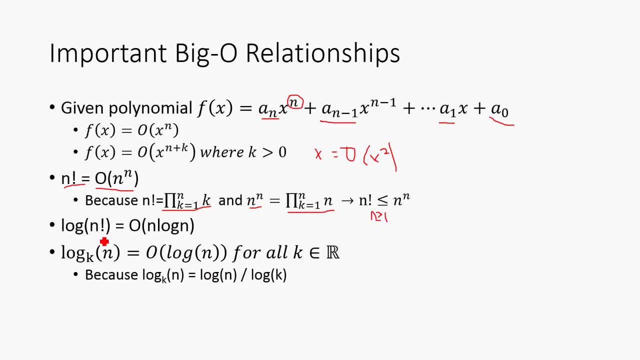 has to hold true right. So consequently, because of this, if we take the log of both sides, we can see that log of n factorial is going to be n log n, And then another really important one is that the log of any base number of n is going to be just big O log n, because the base doesn't. 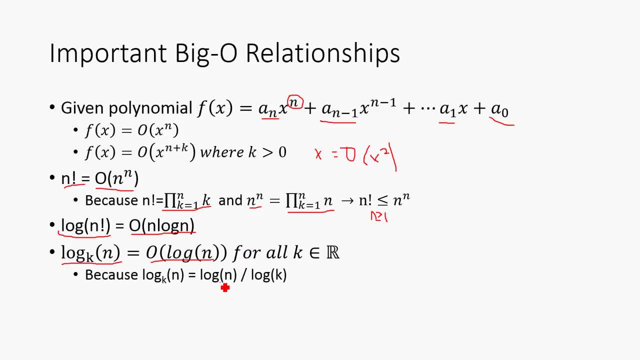 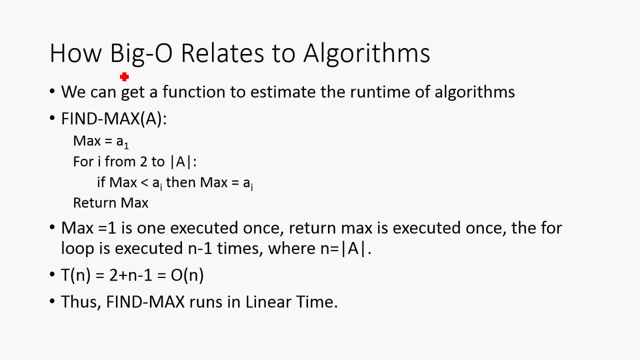 really matter, right, Because we can just change the bases By using a logarithm of any base, right? So let's say this was log base d. It's completely inconsequential, right? So how does this big O relate to algorithms? Well, we can find a function. 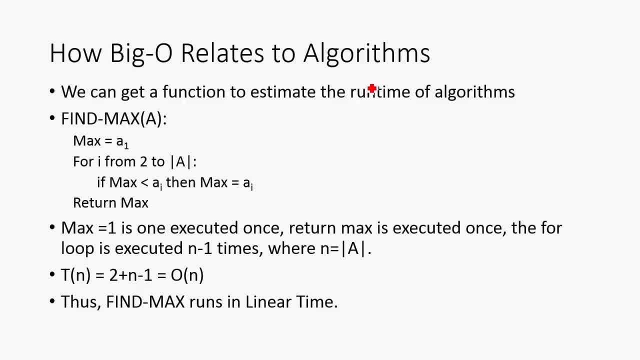 to estimate the running time of an algorithm, and then we can determine its asymptotic behavior from there. So let's take, for example, our find max function. We can notice that this instruction, right here the max equals a A1 and return max. these are both executed once. so these are both what we call big O of 1.. 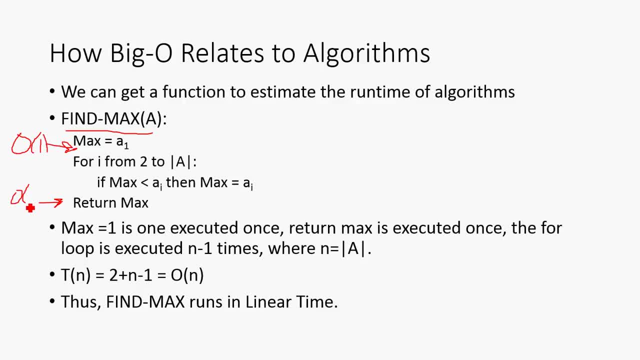 They run in constant time. So then the next piece is this: for loop right here and that runs n minus 1 times right, n minus 1.. Hopefully that's clear, Because it starts from 2, and it goes to the end of a, which is n. 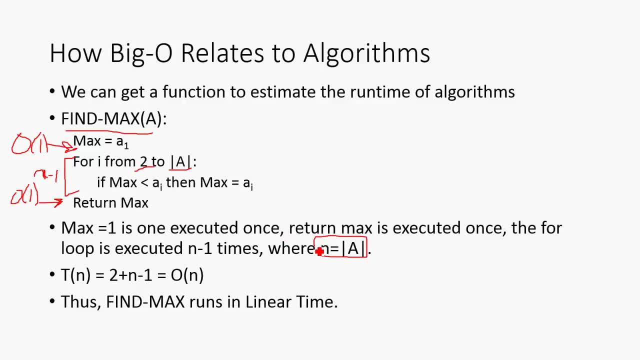 Right. So n is going to be the cardinality of a, so the number of elements in the data structure. So we say that our function that estimates the running time t of n is going to be equal to 2 plus n minus 1.. And this is clearly big O of n from the relationship we saw on the other slide. 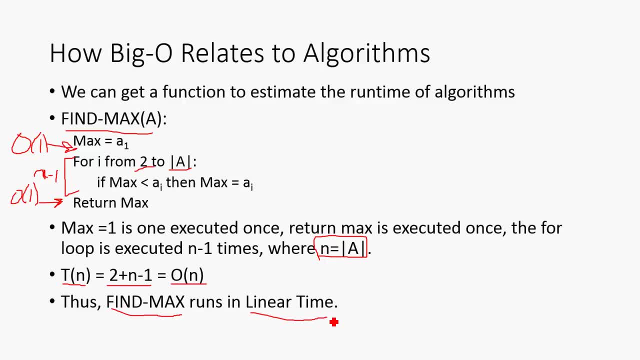 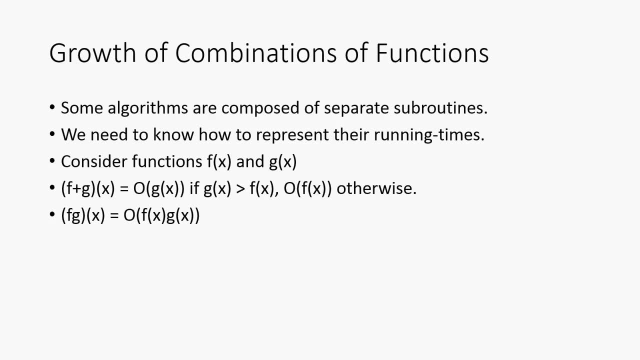 So this find max runs in what we call linear time or big O of n. These two mean the same thing. Sometimes algorithms are composed of separate subroutines or functions within functions. We need to consider how to represent these running times right. So consider functions. 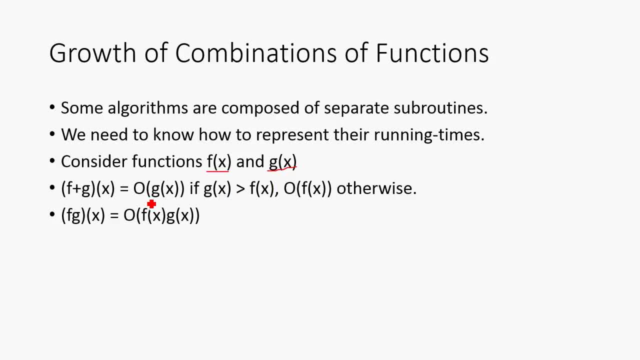 f and g. they're just arbitrary functions. We say that the sum of these two functions is going to be O if g is the bigger one. otherwise it'd be f, which means that that's the bigger one. So it's just O essentially. 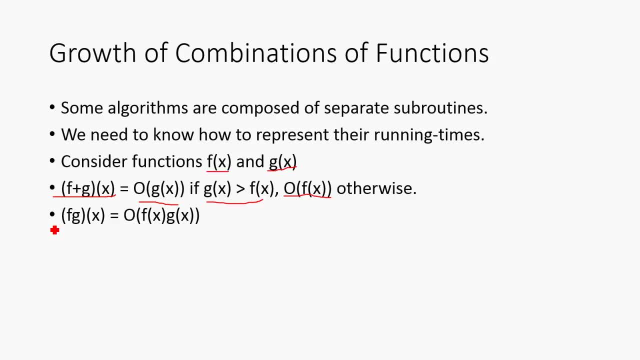 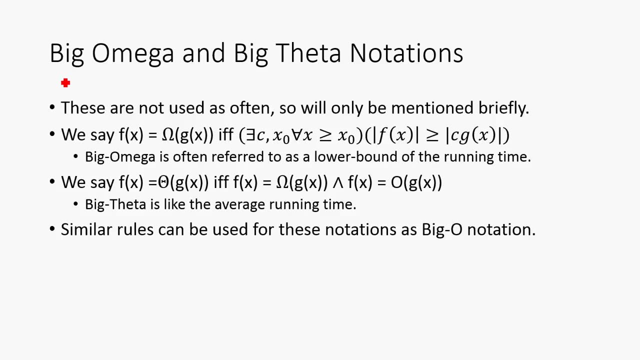 Because it's upper-bound. Then we also have to consider the product. this product of f and g is going to be simply the product …. League O, the product of their running times. So next we have to talk about big-omega and big-theta. 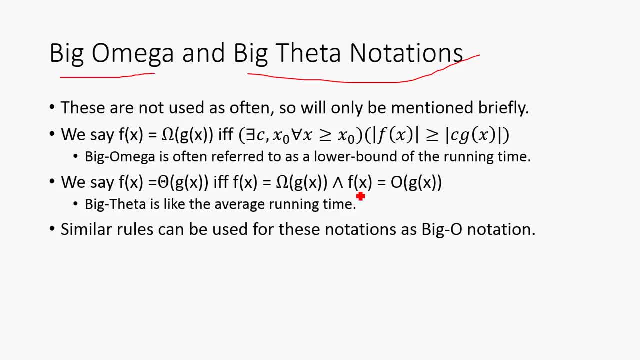 So big-omega is very similar. if you notice from the definition, Everything looks the same except for the direction of this inequality. I noticed that it looks very similar from the definition of big-omega and big-theta around this inequality. It also leaves no trouble to measure the time or length of this lastNew容bert's solution ByForm answer. 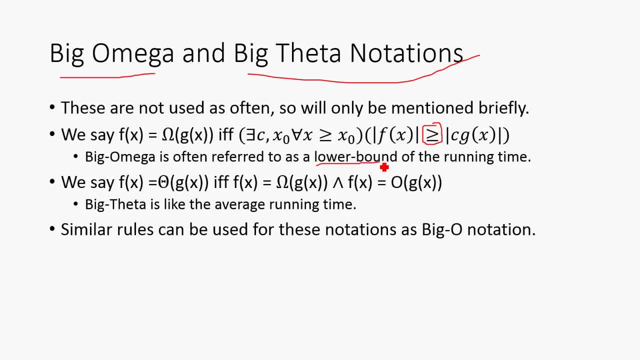 You then have to give a welcoming appearance of big-omega and big-theta, which it believes is right, pointing the other way. that's because it is a lower bound of the running time, right? So same rules apply. this is just the lower bound. And then we also have big theta notation and we say: 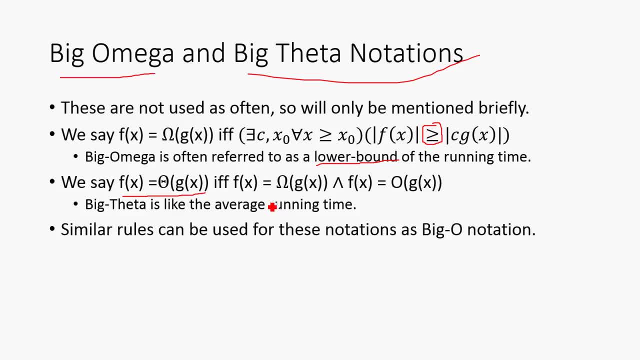 that f of x is big theta of g of x if, and only if, It's both big omega and big O, right? So it has to be omega and O, So it's sort of like the average running time And the similar rules for. 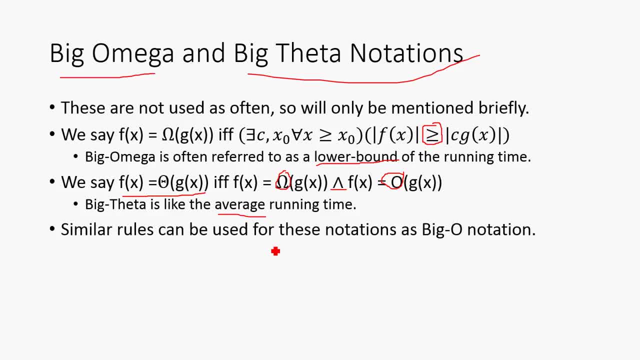 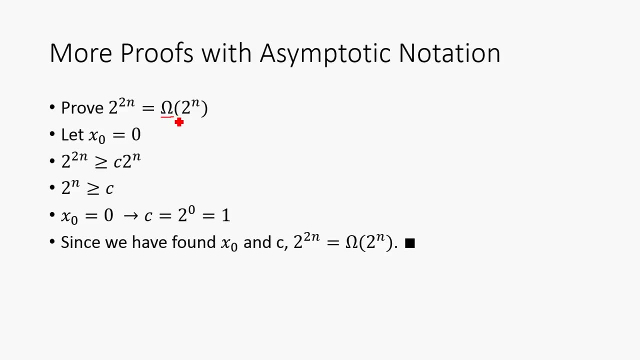 both of these can be used as big O notation, For example. the polynomial relationship that we saw earlier of degree n can still hold for both of these. So then, here's another proof of asymptotic notation. this time we're going to be using big omega, So we're going to start off by letting x.